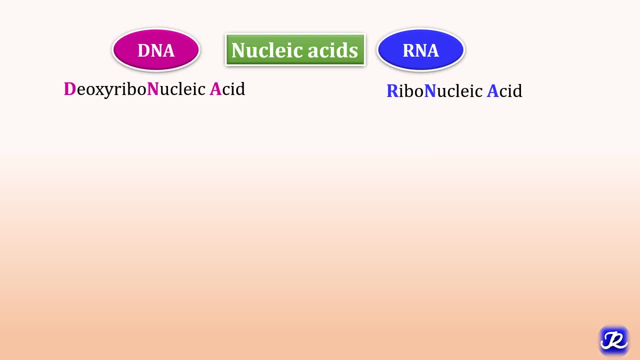 like red roe viruses, The genetic information is passed from one generation to next generation, and RNAs play a crucial role in the process of transmission of genetic information in all species. These nucleic acids: they are polymers of nucleotides And these are also called as building blocks of nucleic acids. These nucleotides are nitrogenous. 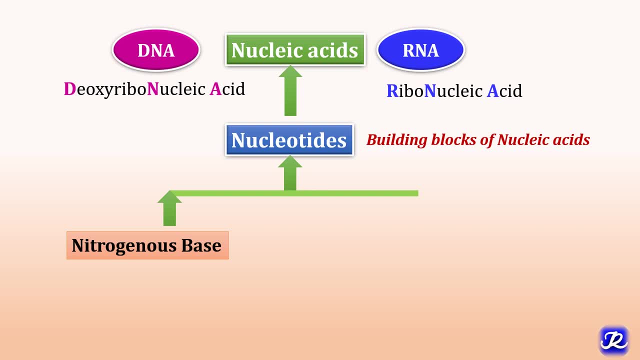 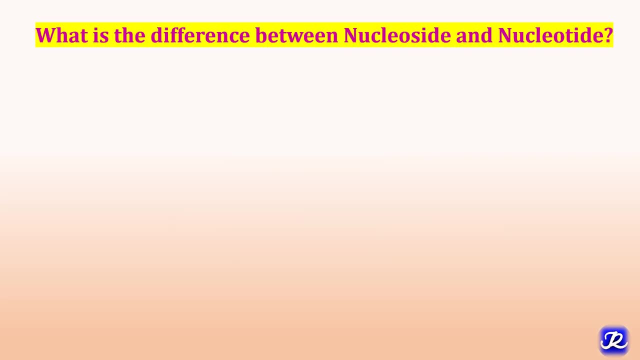 compound. They are consisting of three components. The first is nitrogenous base, second is pentose sugar and third is phosphate. What is the difference between nucleoside and nucleotide? When sugar is attached to nitrogenous base, it is called as nucleoside, and when sugar is attached, 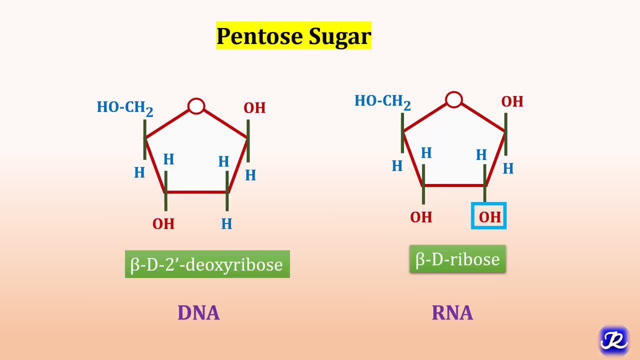 to phosphate. it is nucleotide. Nucleic acids have two kinds of pentose sugar and five carbon atoms of sugar are given prime numbers like 1 prime, 2 prime, 3 prime, 4 prime and 5 prime, Both types. 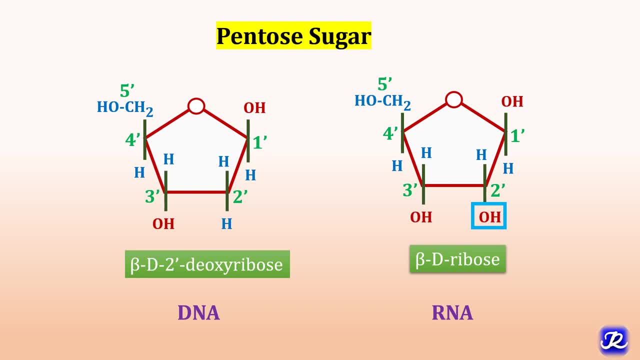 of pentoses are in their beta form. Beta form means hydroxyl group is attached to carbon 1 and it lies above the plane of this cyclic ring. Beta 2 deoxyribose sugar is present in DNA and it is present in DNA. 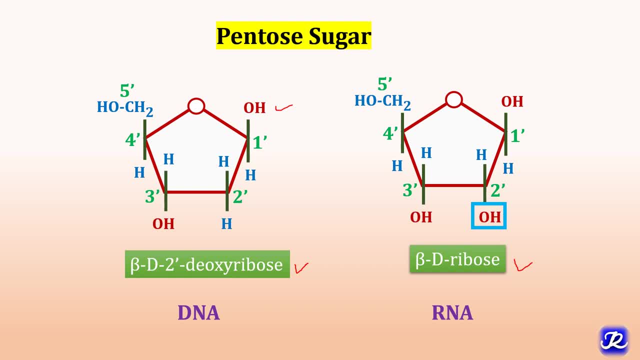 And beta D ribose sugar is present in RNA. The difference between deoxyribose sugar and ribose sugar is that the hydroxyl group present at C2 position is just replaced by hydrogen atom. So in case of deoxyribose sugar at C2 position, only hydrogen atom is present, while in case of 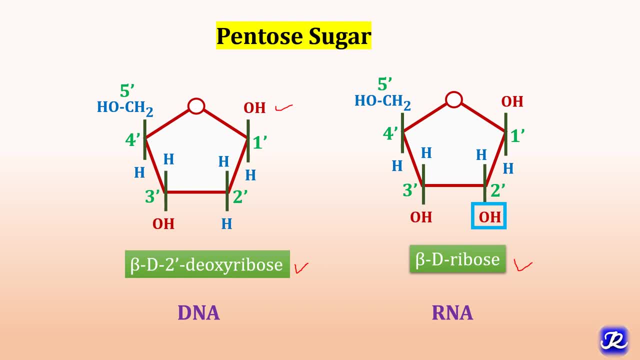 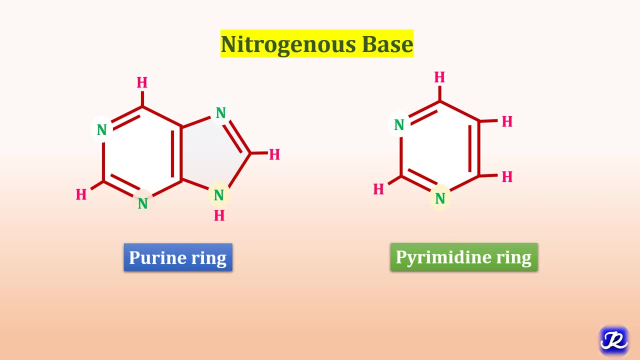 ribose sugar at C2 position. hydroxyl group is attached. There are two types of nitrogen containing bases Commonly found in nucleotides: purines and pyrimidines. Purines are nine membered heterocyclic nitrogenous ring and the atoms are numbered as cardinal numbers, like 1, 2, 3,, 4,, 5,, 6,, 7,, 8 and 9.. 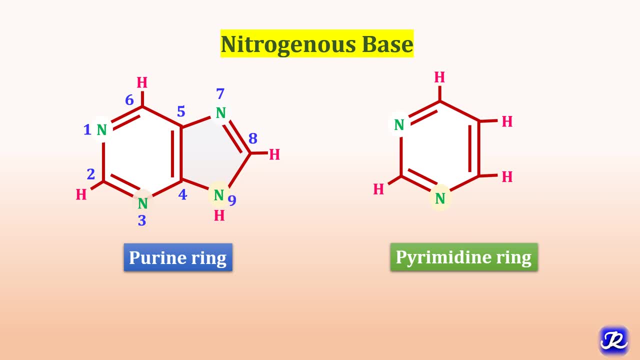 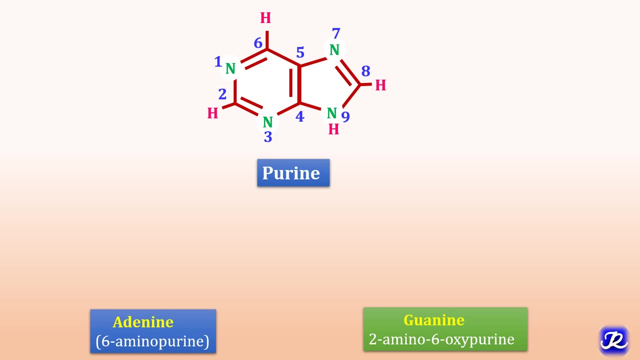 While pyrimidine is six membered heterocyclic nitrogenous ring and it is numbered as 1,, 2,, 3,, 4,, 5 and 6.. Purines contain two rings in their structure, And the two purines commonly found in nucleic acids are adenine and guanine, and both are 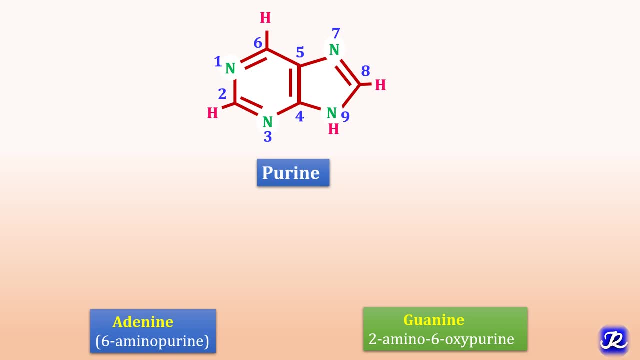 found in DNA and RNA. Adenine is also called as 6-aminopurine, because at the 6th position amino group is attached, and guanine is also called as 2-amino-6-oxypurine, because at the 2nd position amino group is. 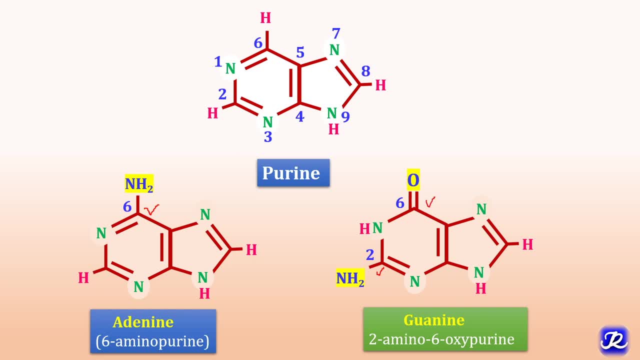 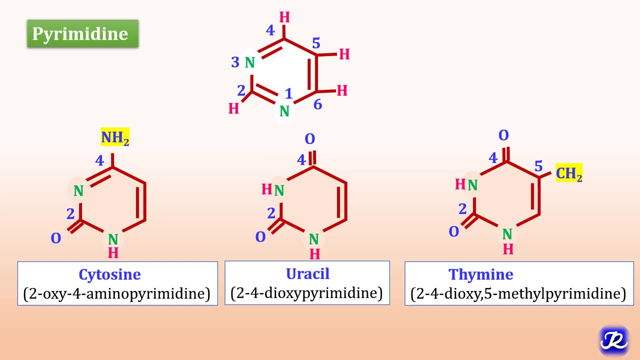 attached, and at the 6th position, oxygen is attached. Pyrimidines have only one ring. There are three types of pyrimidines: cytosine, uracil and thymine. Cytosine is also called as 2-oxy-4-aminopyrimidine because at 2nd position, oxygen is attached. 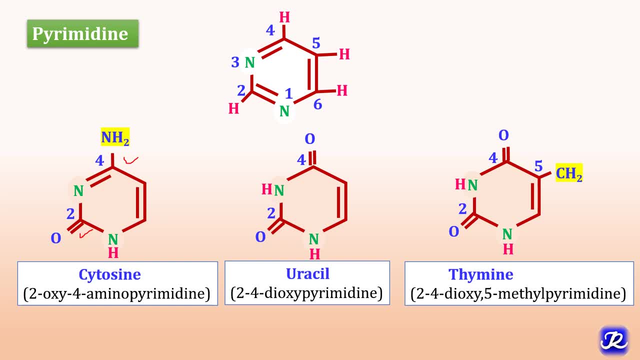 and at the 4th position amino group is attached. Uracil is also called as 2-4-dioxypyrimidine, because at the 2nd and 4th position oxygen is attached, While thymine is called as 2-4-dioxy-5-methylpyrimidine, because at the 4th position oxygen is attached. 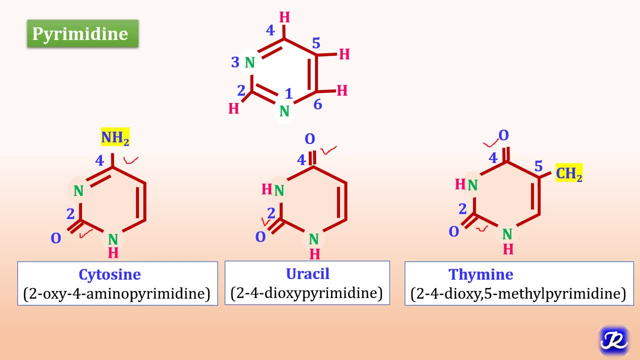 At the 2nd and 4th position, oxygen is attached and at the 5th position, methyl group is attached. Cytosine is present in both DNA and RNA, Uracil is present only in RNA and thymine is present only in DNA. 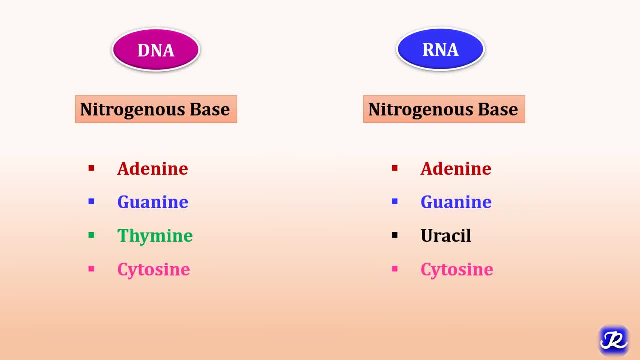 The nitrogenous bases present in DNA are adenine, guanine, thymine, cytosine, and the nitrogenous bases present in RNA are adenine, guanine, uracil and cytosine. Nitrogenous bases are planar in nature and this helps in stacking of bases. one above: 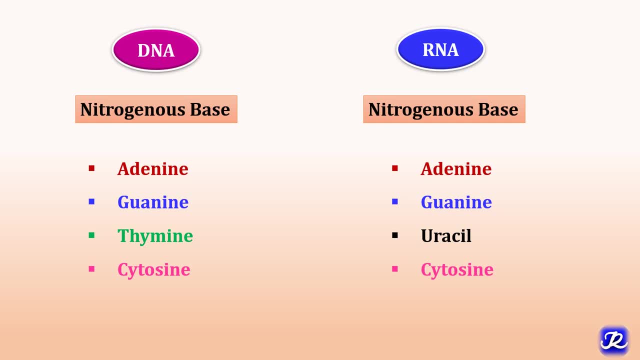 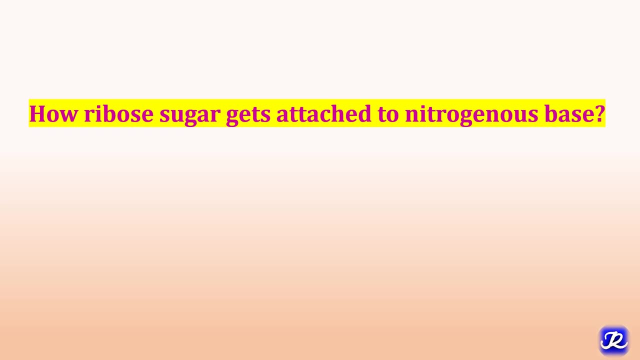 other. This property is helpful in stabilization of DNA structure. Now let's see how ribosugar gets attached to the nitrogenous base. The nitrogenous base of nucleotide is linked covalently to pentose sugar by beta and glycosidic. 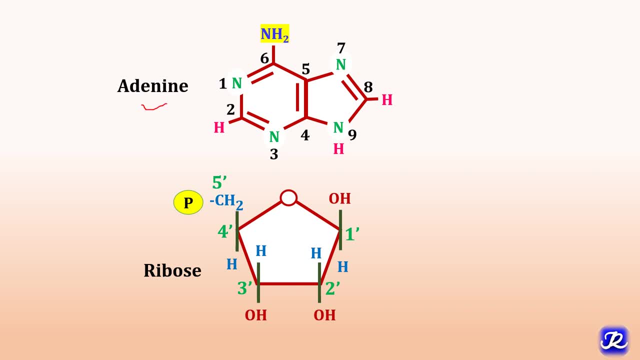 linkage. This is adenine, it is a purine and this is a ribose sugar. Phosphate group is attached at the 5th position. Now let us see how the purine base is attached to the ribose sugar. We can see here: at the N9 position the hydrogen atom is present and at the carbon 1 position 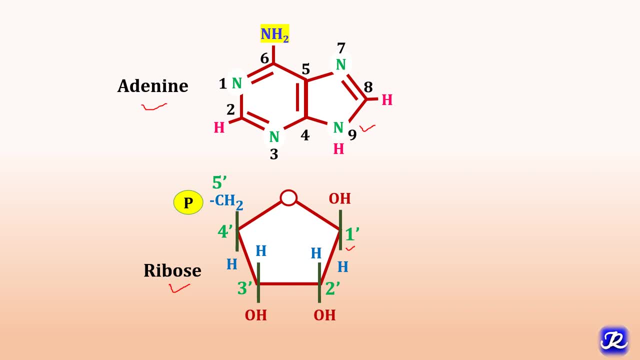 in sugar hydroxyl group is present, So beta and glycosidic bond is formed between this N9 and C1 and there is removal of hydrogen atom from adenine and hydroxyl group from ribose sugar to form a water molecule and 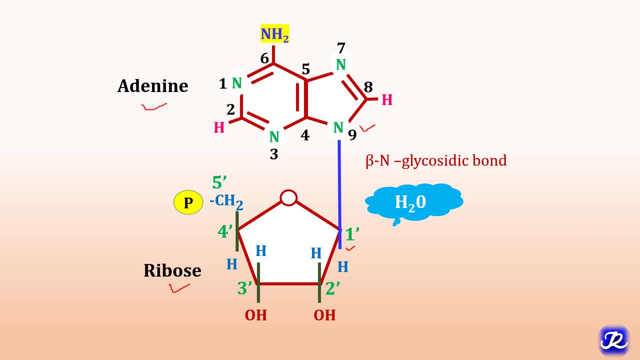 beta and glycosidic bond is formed between this N9 and C1. So beta and glycosidic bond is formed between adenine and ribose sugar, and the structure is called as adenilic acid and or adenine ribonucleotide. 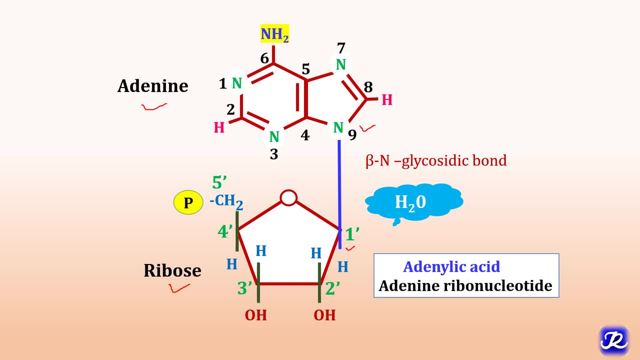 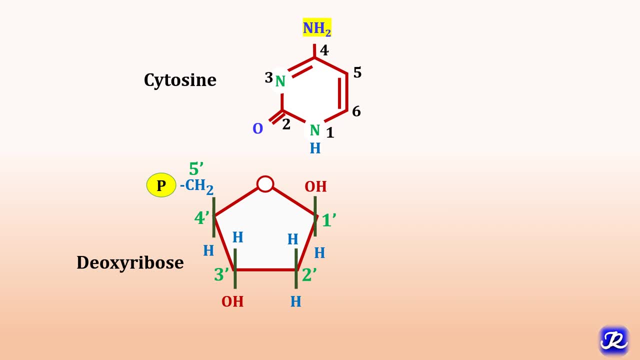 As one phosphate group is attached, it is also called as adenosine monophosphate. Now let's see how glycosidic bond is formed between pyrimidine and pentose sugar. This is cytosine, which is a pyrimidine, and this is deoxyribose sugar. 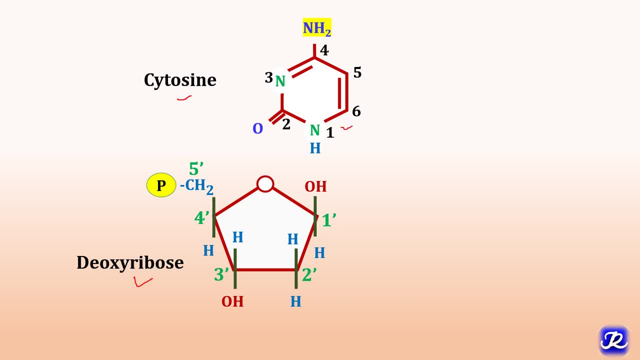 So at N1 position of cytosine, Which is a pyrimidine hydrogen group, is attached, and at the C1 hydroxyl group is attached in case of deoxyribose sugar. So the beta and glycosidic bond is formed between N1 of pyrimidine and C1 of pentose sugar. and 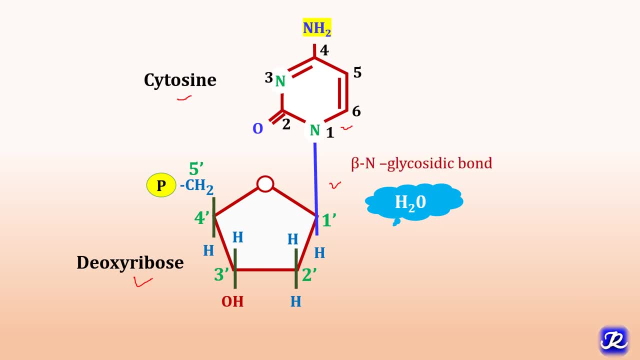 there is removal of water molecule and beta and glycosidic bond is formed, and it results into deoxycitadilic acid, which is also called as cytosine deoxyribonucleotide. The important question is why DNA does not contain uracil. 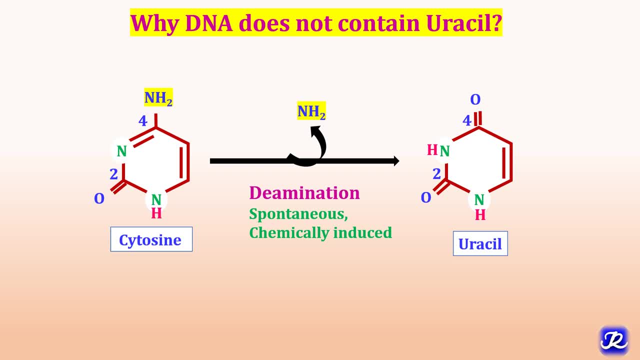 Cytosine is a pyrimidine which undergoes spontaneous as well as chemically induced reamination, and it leads to formation of uracil. Therefore, under such conditions, DNA shows uracil and not cytosine. Had uracil originally present in DNA, it would have been difficult to determine whether a given uracil has a 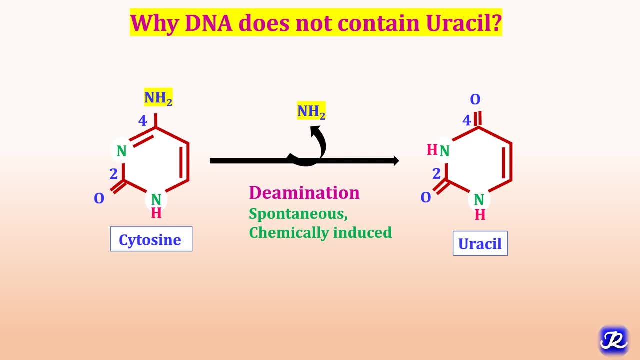 horizon from cytosine by its deamination, or it was originally present in the DNA sequence. Hence, during evolution, uracil is lost and it is not present in DNA. Now it is very clear that if it is present in DNA, it is a sign of mutation and it is 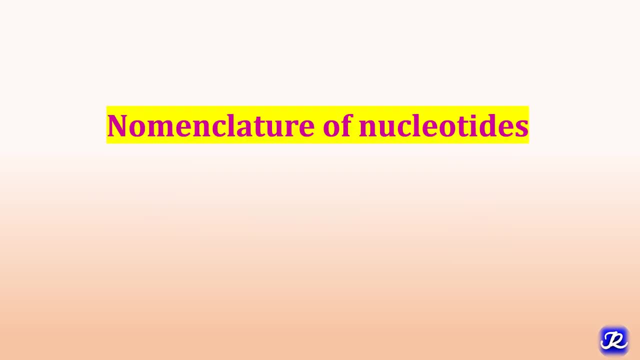 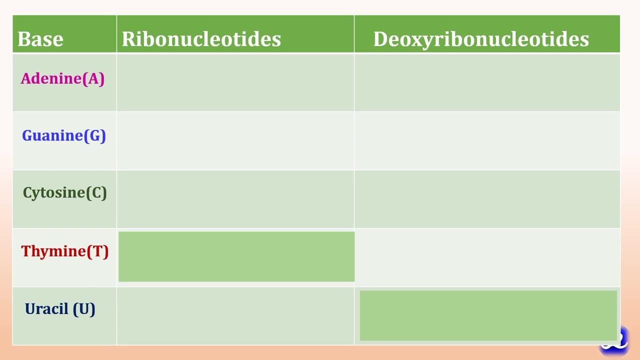 removed by repair mechanism. Now let's see the nomenclature of nucleotides. Adenine is a purine which is present in both RNAs, So ribonucleotide form of adenine is adenosine, monophosphate, AMP or adenilic acid. 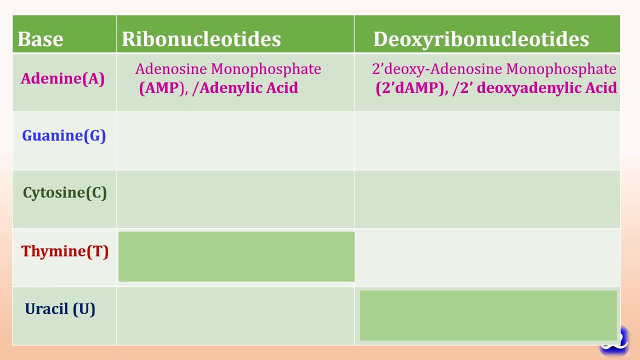 Deoxyribonucleotide is 2'-deoxyadenosine monophosphate, 2'-DAMP or 2'-deoxyadenilic acid. Gonine is a purine which is also present in both DNA and RNA. 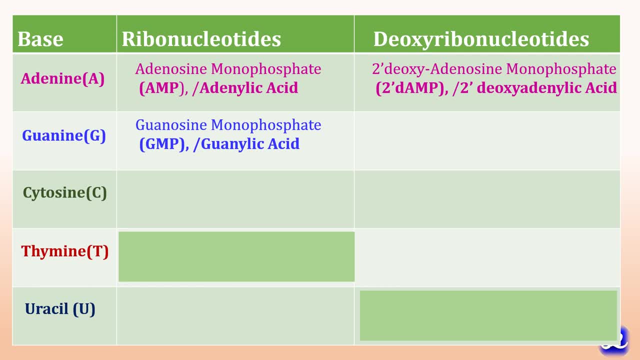 The ribonucleotide is gonosine monophosphate, GMP or gonilic acid, And 2'-DAMP or 2'-DAMP Deoxyribonucleotide is 2'-deoxygonosine monophosphate or 2'-DGMP is a deoxyribonucleotide. 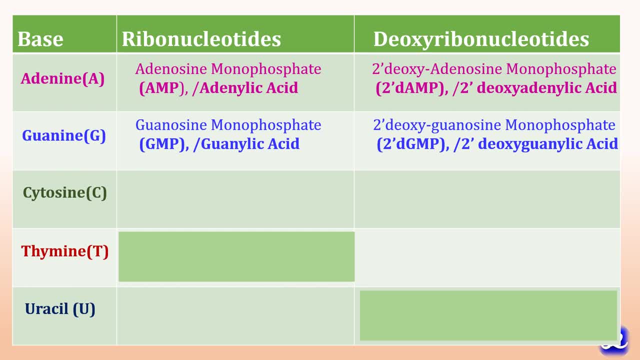 It is also called as 2'-deoxygonilic acid. Cytosine is a pyrimidine which is present in both DNA and RNA, And the ribonucleotide is cytidine monophosphate, CMP or cytidilic acid. 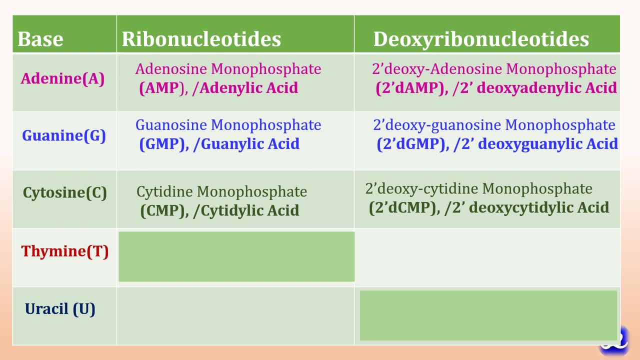 And deoxyribonucleotide is 2'-deoxycytidine monophosphate, 2'-DCMP or 2'-deoxycytidilic acid. Thymine is present only in DNA, so it is present in the deoxyribonucleotide form, that is, 2'-deoxythymidine. 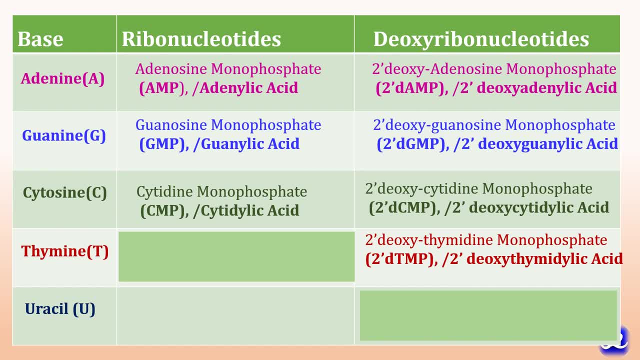 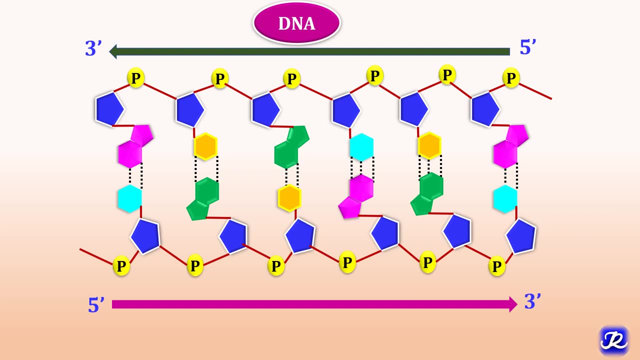 monophosphate or 2'-deoxythymidilic acid. Uracil is present only in RNA as a ribonucleotide, that is, uridine monophosphate, UMP or uridilic acid. So let us summarize: DNA is deoxyribonucleic acid. it is double standard structure. 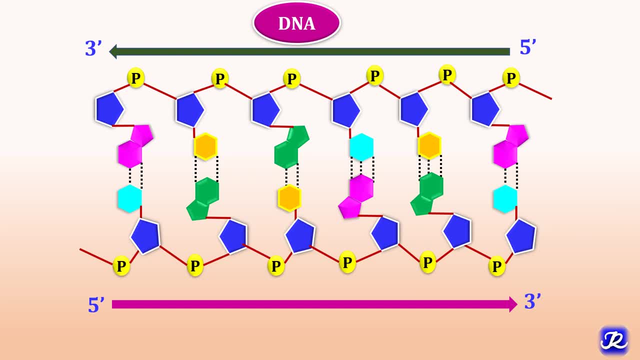 It is a polymer of deoxyribonucleotides which contains deoxyribosugar. It has four bases- adenine, guanine, cytosine and thymine- and it also has a phosphate group. It is a storage of genetic information. 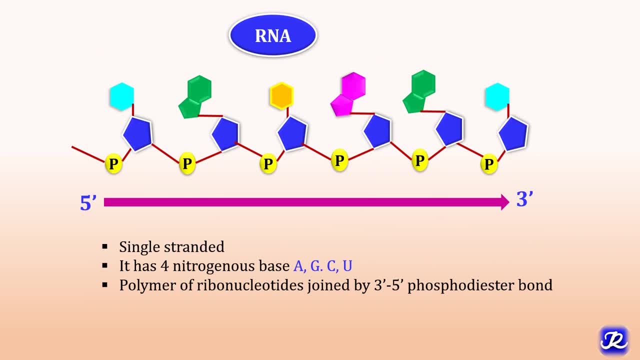 RNA is a ribonucleic acid. it is single standard. It has four nitrogenous base: adenine, guanine, cytosine and uracil. It has ribosugar and it is polymer of ribonucleotides which are joined by 3'-5' phosphodiester.